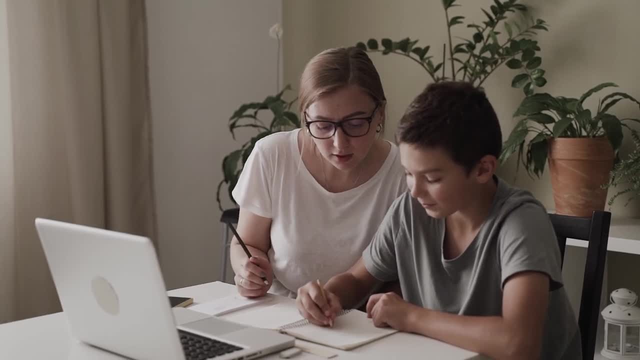 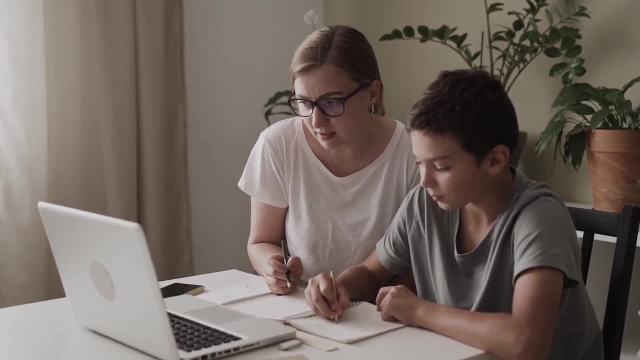 and show how you compare brands to make your money buy more. When your child wants to buy something with her allowance or money she's been saving, show her how to comparison shop with online sales circulars and by checking store websites for prices so she can get the most for her money. 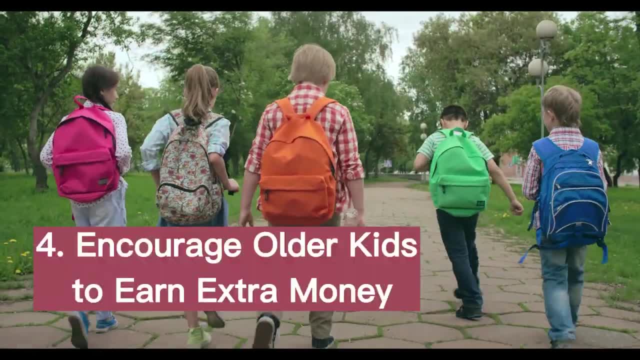 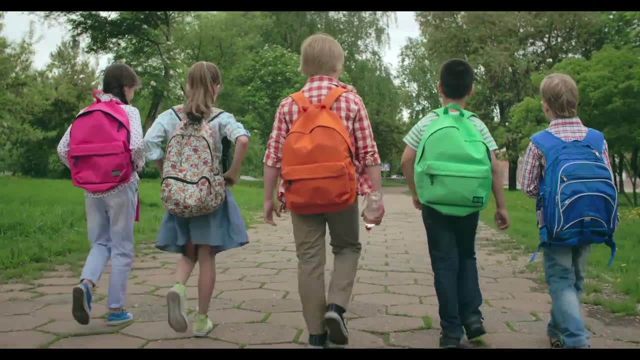 4. Encourage older kids To earn extra money. Middle schoolage kids may not be eligible to get a traditional job, but that doesn't mean they don't have opportunities to earn extra money. Here are some ways kids can earn a little extra. 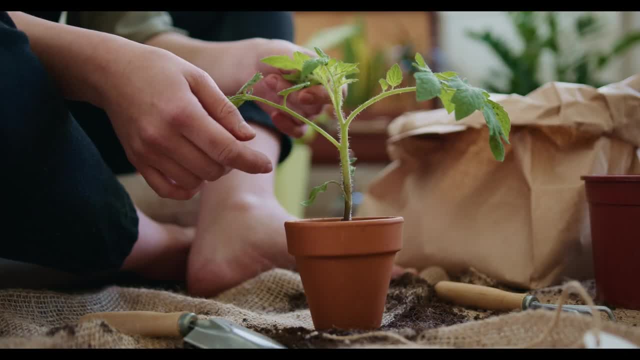 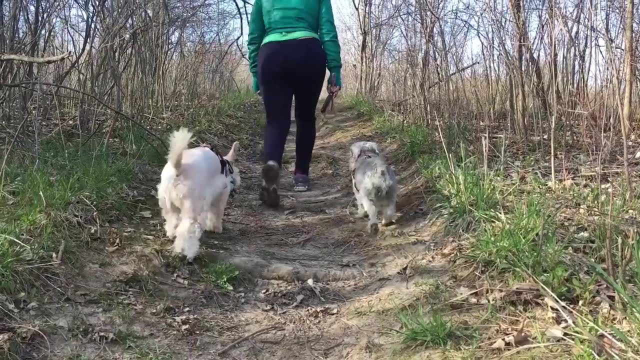 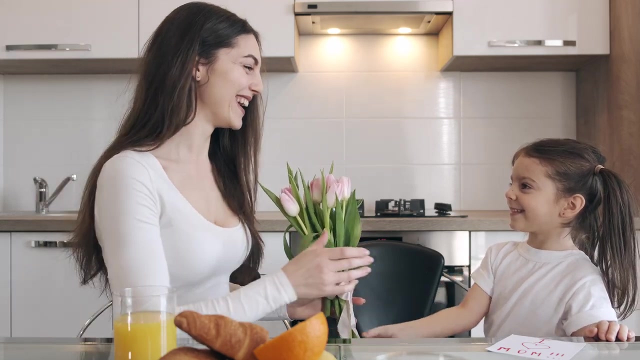 Collecting recyclables and taking them to the recycling plant. Organizing and setting up a family garage sale. Doing yard work in summer and snow shoveling in winter for neighbors. Day-besitting, Doing housework for elderly or infirm neighbors, Tutoring students who are struggling with academic subjects. 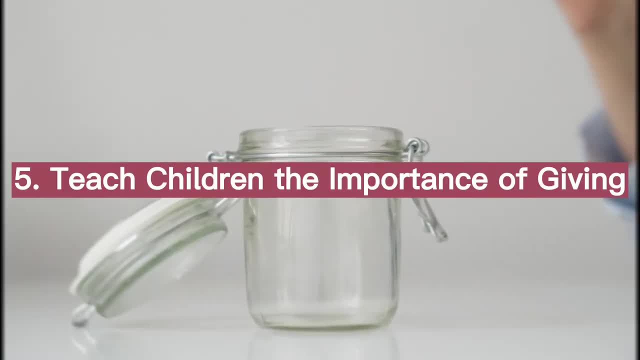 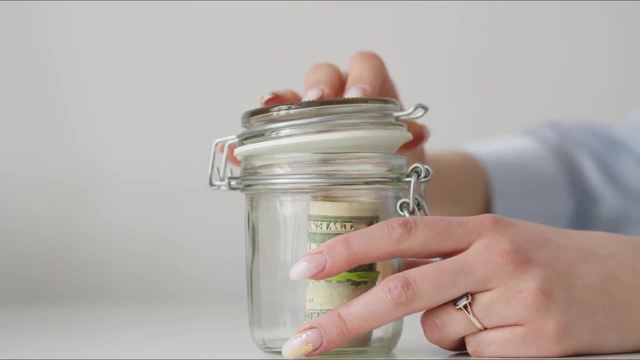 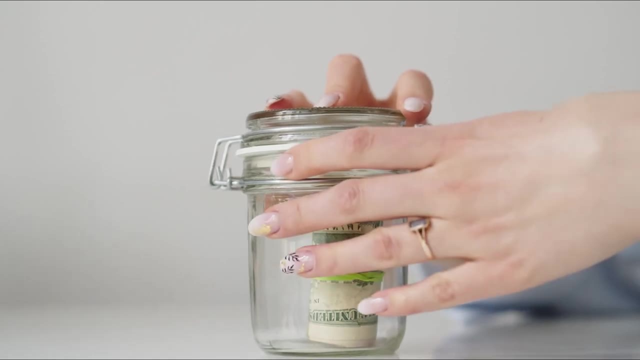 Tetsitting and dog walking. 5. Teach children the importance of giving. While earning, saving and spending are important, so is helping out those less fortunate. Explain to your kids why you give money to charity and encourage them to give some of their allowance or other earnings to the less fortunate. Learn about what your child feels. 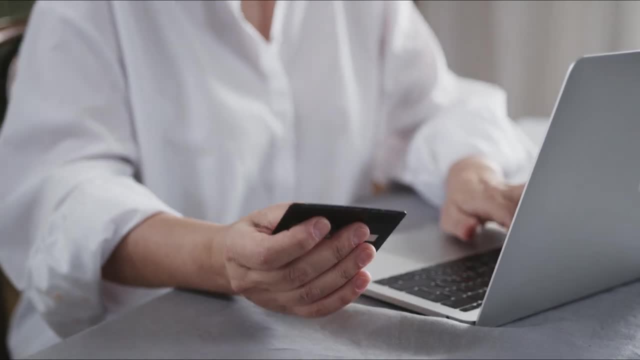 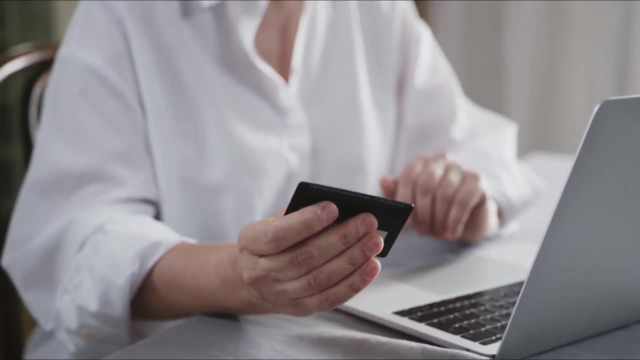 strongly about and share with your friends and family. Learn from your kids what you can do to help them make money and show them ways to help if they love animals, for instance, help them raise money for a local animal shelter. children should understand that giving their time is an important way to help. 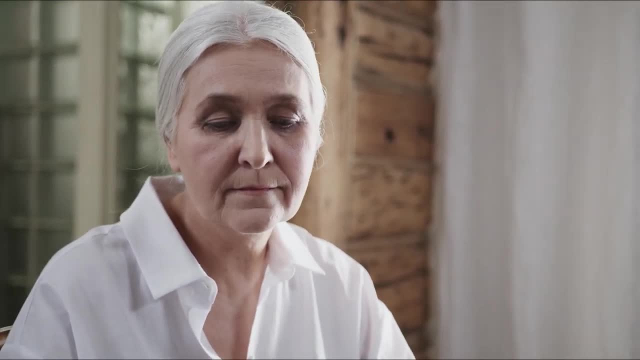 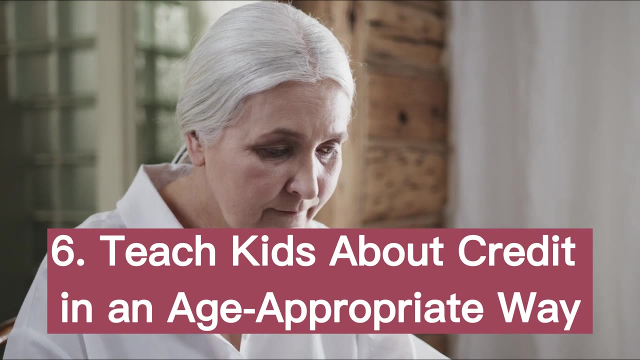 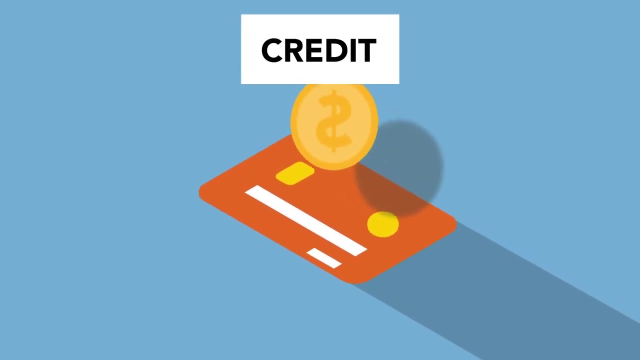 others when they don't have a lot of money to donate. six: teach kids about credit in an age appropriate way. when your middle schooler wants to buy something that's relatively expensive, tell them they can save up or borrow the money from you with interest and a loan due date if they fail to pay you back on time. 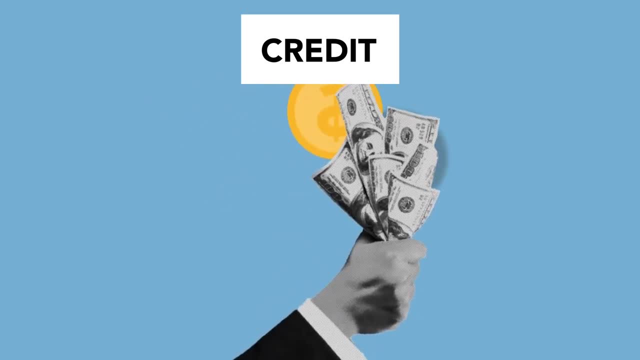 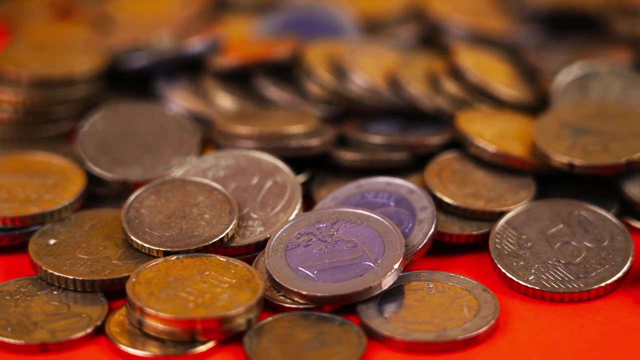 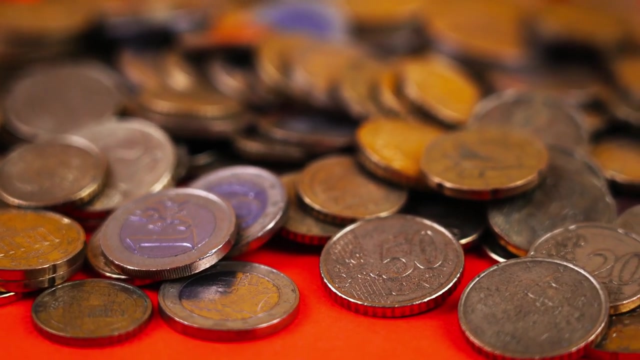 show them the consequences by adding a penalty cost. money management is one of the most valuable life skills you can teach your children, and starting when they're young is best. demonstrating good money management yourself is extremely important because kids are so good at absorbing what's going on around them.